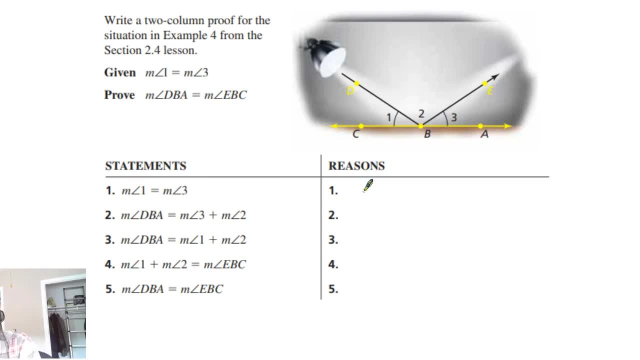 statements. we just got to come up with the reasons, And that's something that you're going to practice Now. one of the things that I I'd like to say in my videos is that I would love for you to hit pause and try to get the 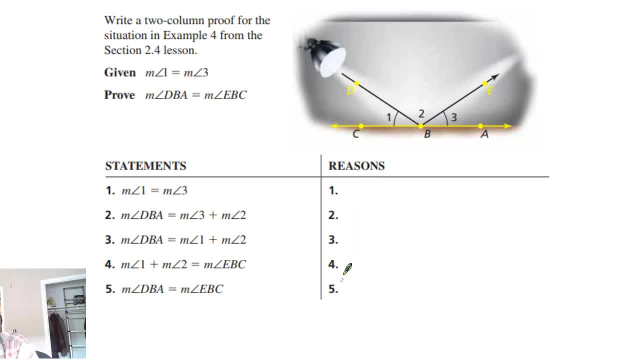 answers before me, And I'd like you to do that for each step along the way. So even if the for the first three, you, you, you need my help if you can hit pause before I give the next reason and then try to give the the extra ones Now, if you can't do. 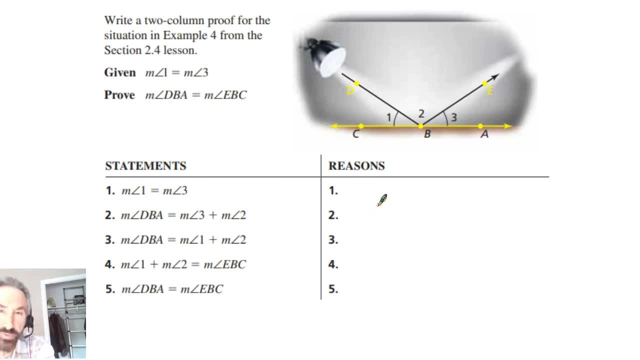 it now, later on, when you're going back and you're reviewing for the test, a good idea would be to try to watch this video. Hit pause at this point and try to fill in all the reasons yourself and then watch me and see if we agree. Okay, anyways, let me get started. So angle one, the measure of 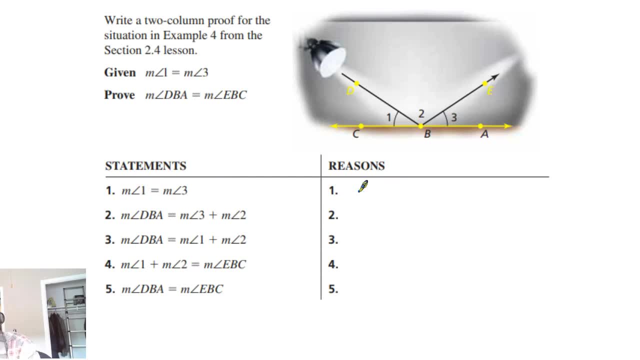 angle one equals measure of angle three. I'm going to say that that is given. Now, sadly, my handwriting is a sloppy mess, but but I'm going to try my best anyways. So next thing: angle: measure of angle DBA is equal to measure of angle three plus two. Here's. 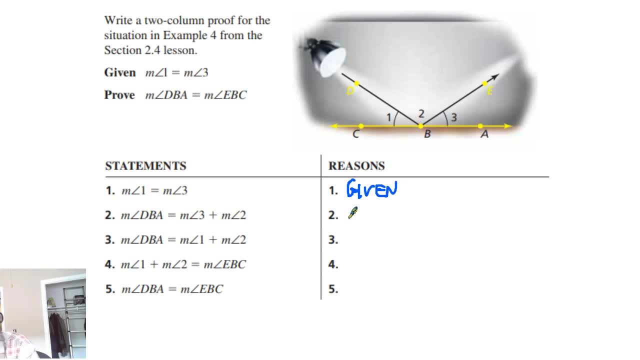 the DBA. Sure enough, it's three plus two. I'd say that would be the angle addition postulate, so something like that: Ooh, let's, let's, let's do this. I'm going to abbreviate angle. 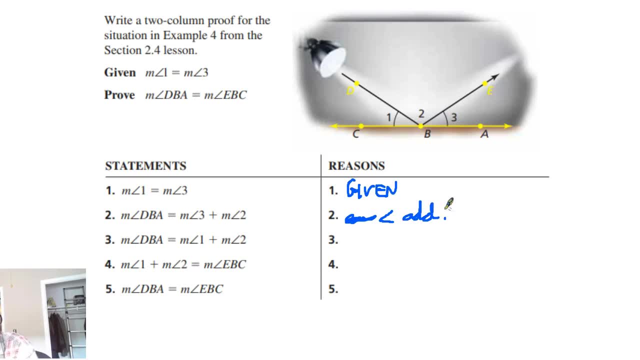 addition. There we go, Something like that, And then I, if you know, if we putting the postulate part is great, but I don't even know that I need it. Angle addition is what you guys need to know. 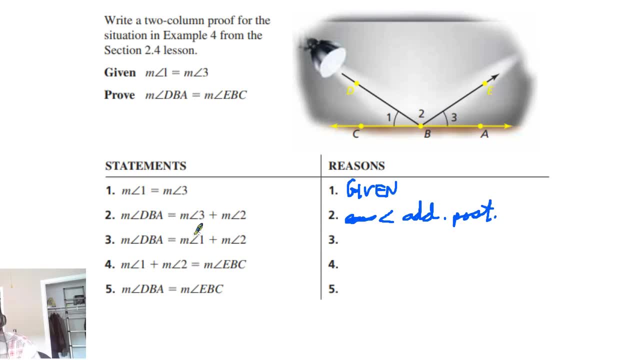 Okay, next Angle DBA is equal to angle one plus angle three, Angle two. let's take a look: DBA Hm. I see two and three, but I don't see angle one and two. But what I notice here is that all they're doing is they're rewriting this, this. 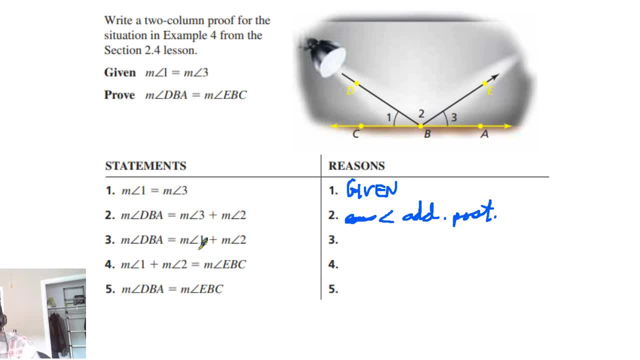 statement for two, and they've replaced the angle three with angle one. Now, is that reasonable? Let's take a look. Well, here's angle three, here's angle one. One of the things we talked about is, if these angles were congruent, they'd have a little hash mark that indicates that. 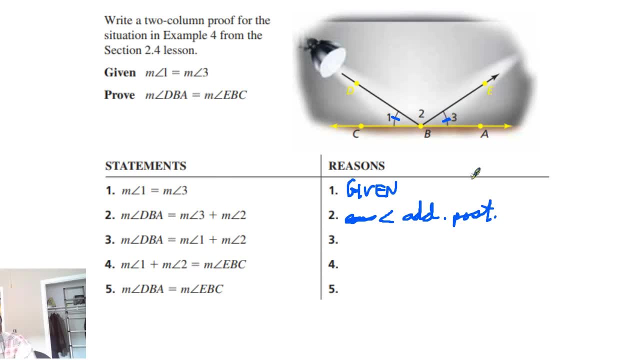 they are the same angle. But there is another way to determine whether angles are congruent or not, And that is when you have the same number of arcs. So, for instance, if we had two angles that were exactly equal to each other. I'm just going to try to do my best. 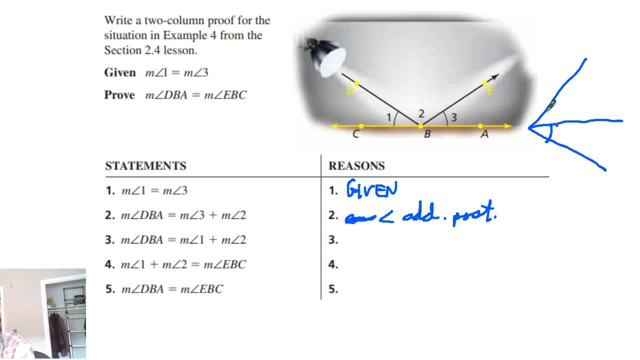 We could. we could say that this angle is equal to this angle by putting the same number of arcs for for the two angles. In this case, since the two angles are congruent, I'm going to say that if there's just one arc here and one arc here, it indicates that these two 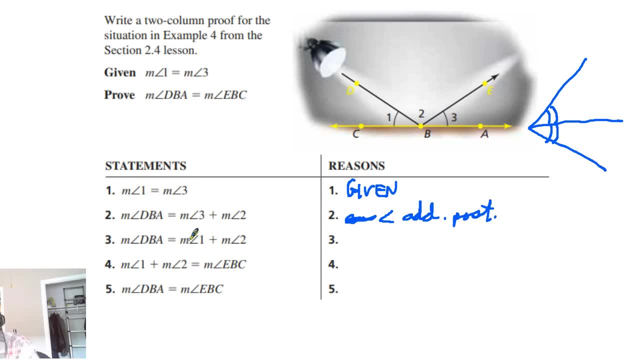 angles are equal. So back to this. Statement three is just statement two, with angle three being placed by angle one. Now why don't you hit pause and see if you can figure out what to write here, and then I'll tell you in just a second. So I believe that we're 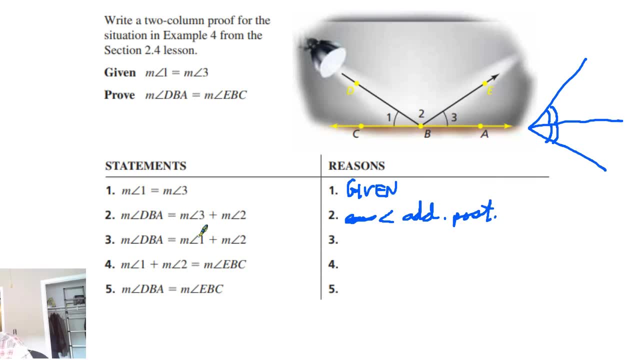 going to say that we can replace the angle three with angle one, because their equivalent will will, oh, and, by the way, it's given that, oh, it's given that angle one is an angle three. So, gosh, we, we could almost say given, but I'm going to say substitution, So I'm going. 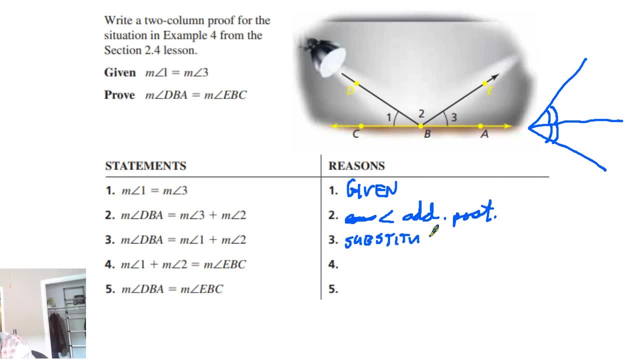 to go ahead and write it in there, And for me I don't know, it's just easier to write in caps. I'll let you write it however you want. Next, it says: angle one plus angle two equals EBC. So here's EBC angle one, two. sure enough. Again, it's just the angle addition. 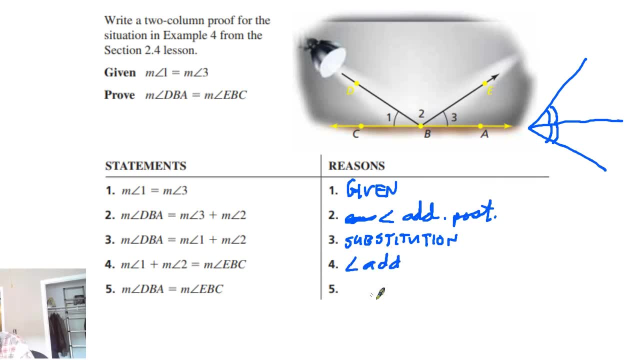 postulate: Oops, sorry about that, I was a little too hasty and I stole your joy. You can go ahead and hit pause and see if you can figure out what to write in there. So I'm going to go ahead and hit pause and see if you can write the last one, And if not, 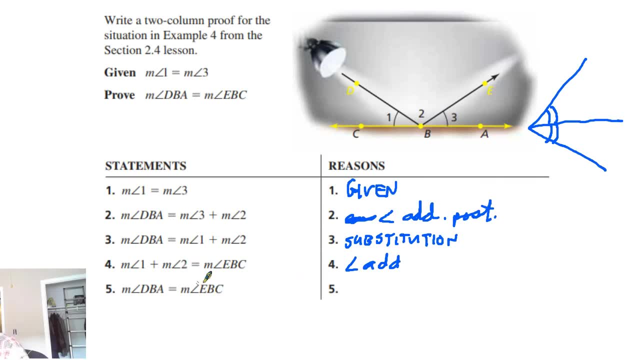 I'll tell you in just a second. Okay, DBA equals EBC. So hopefully you took some time and stared at all of this for a little bit and kind of came up with some thoughts of your own. If you haven't again hit pause and do that, Okay, Now I have some thoughts.